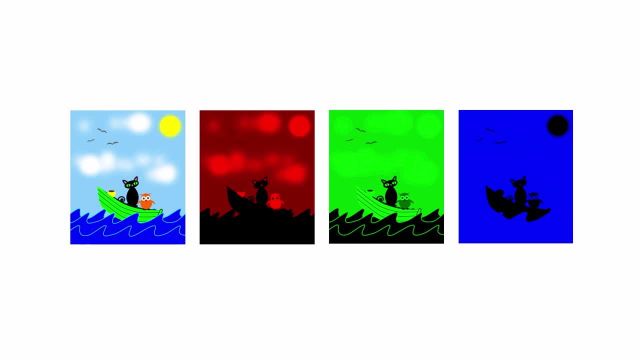 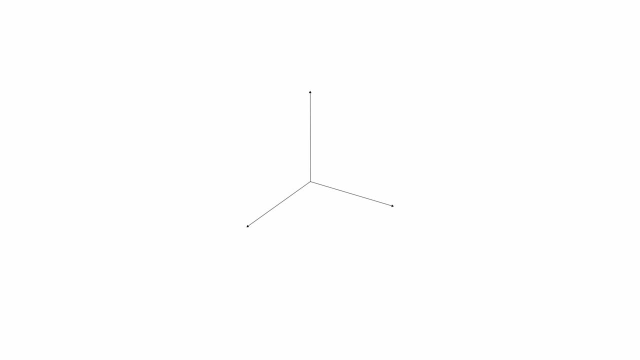 between 0 and 255.. It's possible to visualise every possible combination of red, green and blue on a three-dimensional chart – a chart which has three mutually perpendicular axes, one for each of the primary colours and with the values on each axis. 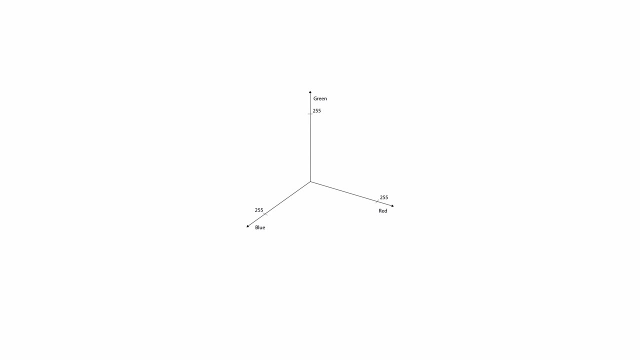 ranging from 0 to 255.. For example, these three particular values of red, green and blue intersect at a point in this three-dimensional chart. You can therefore imagine that every possible colour is located somewhere within this cube. This cube represents the full range of colours possible with the 24-bit RGB system or to 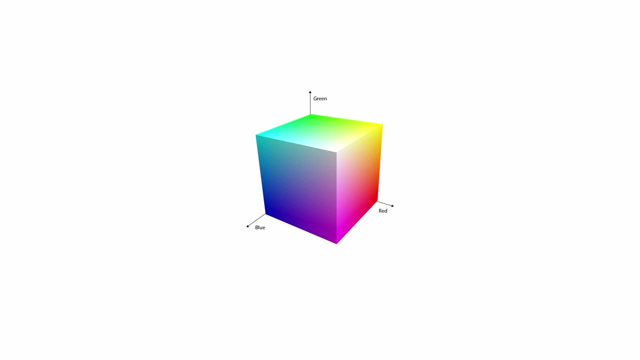 put it another way, this cube represents the full gamut of the RGB colour space. Notice that the nearest top corner of this cube is white. This is where the values of red, green and blue are all at their maximum of 255.. When the same cube is viewed from the opposite side, you can see the origins of these three. 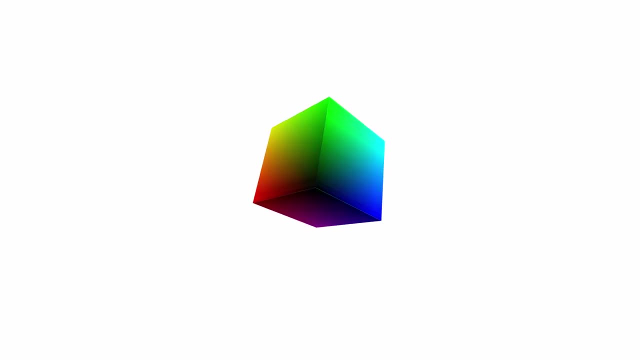 axes – the point at which the values of red, green and blue are zero. This is where you'll find a complete absence of colour – namely black. If we increase the three values for a pixel, or indeed any one of them, the values of red. 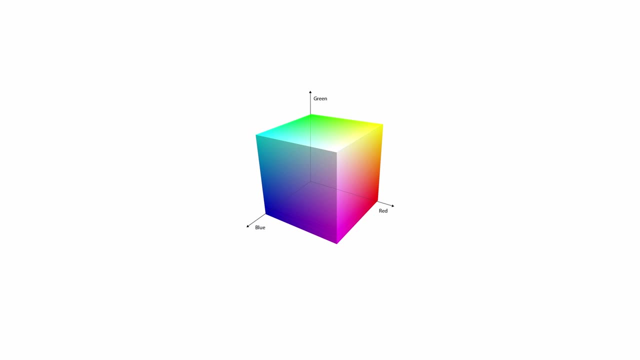 green and blue are at their maximum, we are necessarily moving closer to the white corner, So it follows that we're increasing the brightness of the pixel. This means that the red, green and blue values for any given pixel inherently contain information about the brightness of. 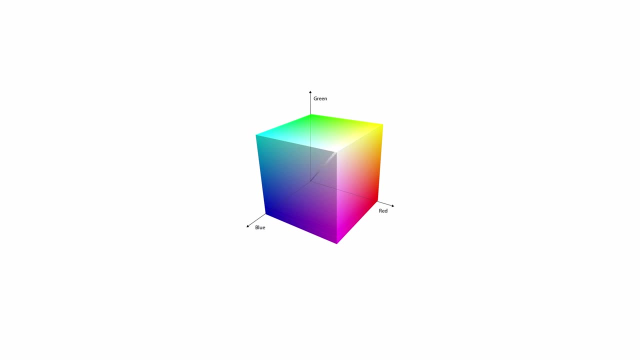 the pixel. Now you can imagine a line connecting the black corner to the white corner of this cube. It's along this space diagonal that you'll find shades of grey – the so-called greyscale. At any point on the greyscale, the corresponding values of red, green and blue are always. 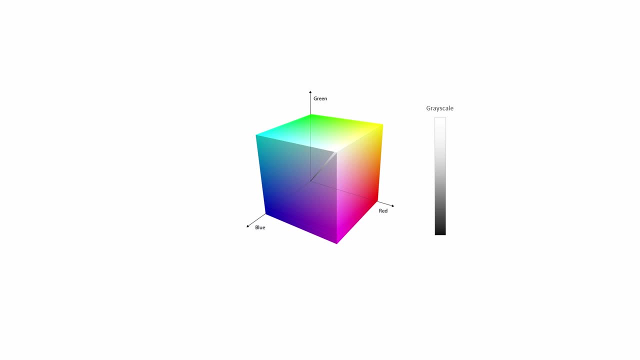 the same as each other. With 24-bit RGB we can encode 16.7 million different colours, but the human eye can only distinguish about 10 million different colours, so the RGB system is not the most efficient way to save or transmit images. 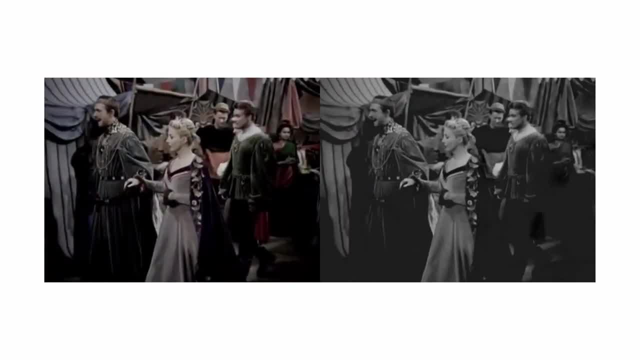 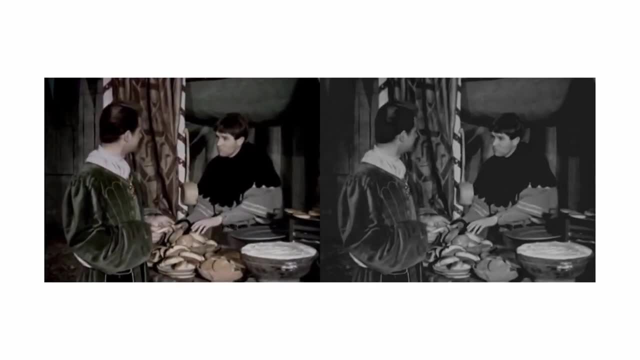 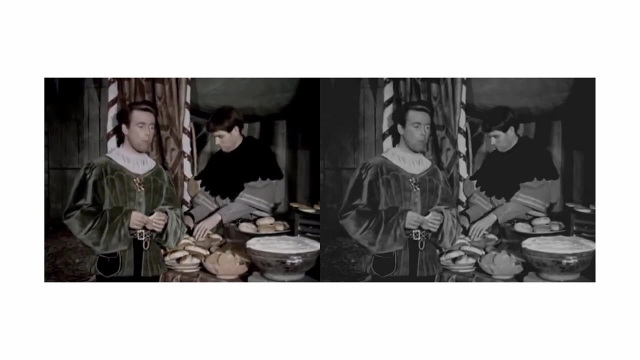 Why CBCR is an alternative to RGB. It evolved from a system known as YUV, which was developed in the 1950s to transmit analogue colour television signals. whilst maintaining backwards compatibility with black and white TV sets, YUV had the added advantage of consuming less bandwidth than RGB would have needed. 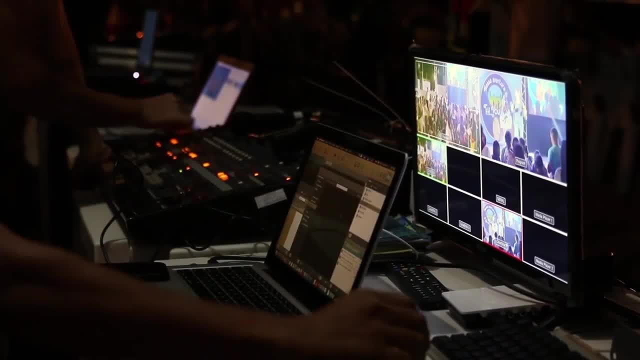 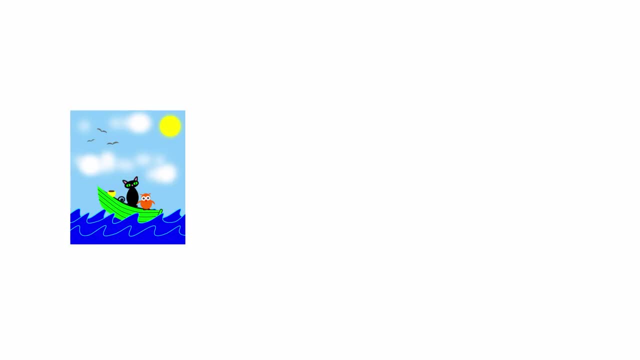 These days. why CBCR is used to store, process and transmit digital TV and video Like RGB. why CBCR uses three separate pieces of information for each pixel, but this information is somewhat different. Y is known as the Luma component. 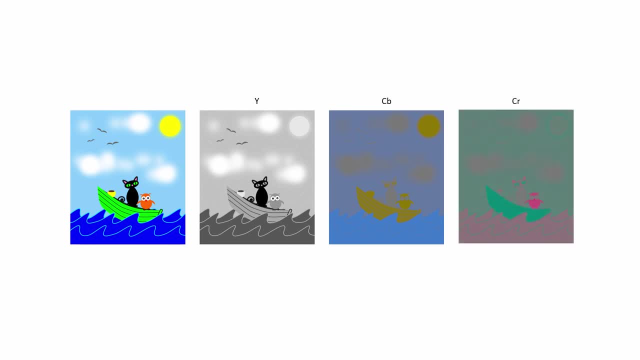 It contains a value for the luminance or brightness of the pixel. This is very similar to the greyscale version of the original image. CB and CR are known as the Chroma components, chroma being the Greek word for colour. CBCR is the chroma component. 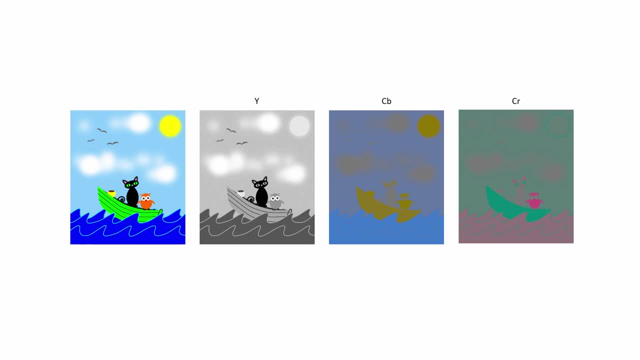 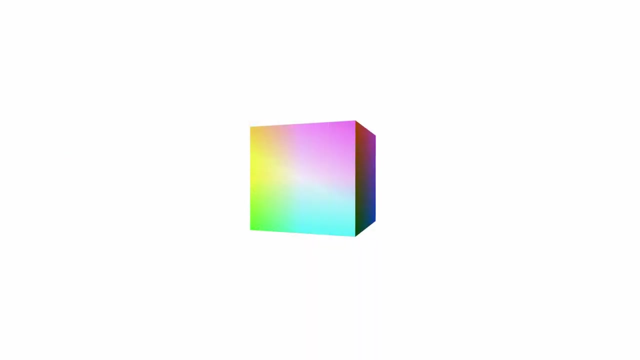 CBCR is the chroma component. CBCR represents the chromonaut's blue component. CR is the chromont's red component. The YCB and CR values for a pixel can be calculated from the RGB values using special formulas. The YCBCR colour space can also be visualised in 3 dimensions. 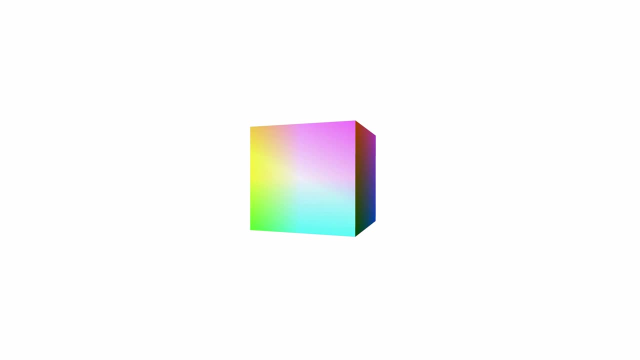 The centre of the face of this YCBCR cube is white. The centre face is black. now imagine a line through the cube connecting the centers of these two faces. this line represents the full range of the luma component Y. or to put it another way, this is the gray scale in the Y, C, B, C, our color model, every. 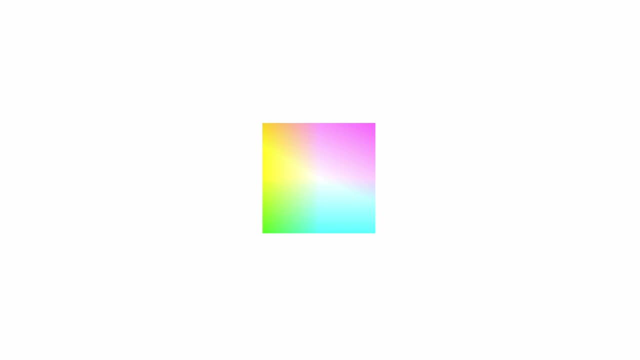 possible value of Y can therefore be thought of as being located in the center of a thin slice of this cube, and the corresponding values of C, B and C R are the coordinates on this two-dimensional chrominance plane. notice that lower values of C, B and C R are in the lower left-hand corner of.